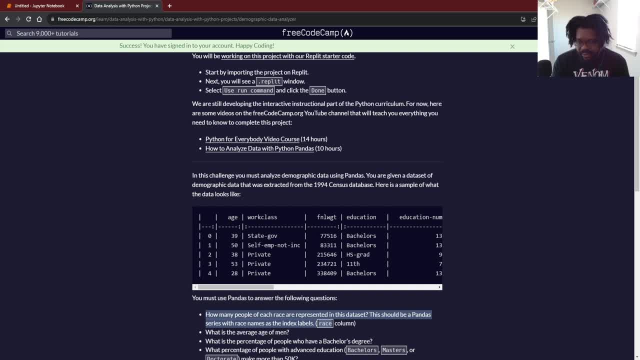 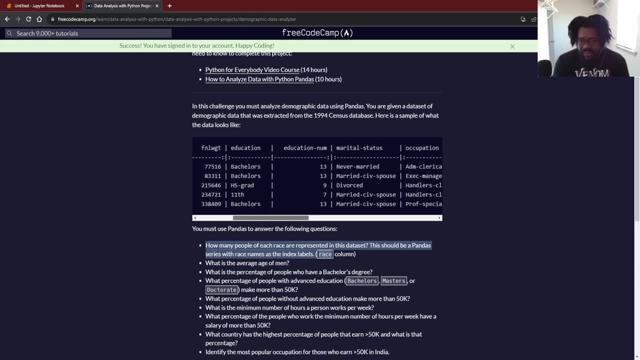 that was extracted from the 19- excuse me, 1994 census. and then this is an example of what it looks like. so we have the age, the work class, the weight, our fnl, wg- i don't know what that is- the education, the education number, the marital status and a bunch of other stuff. so this is the 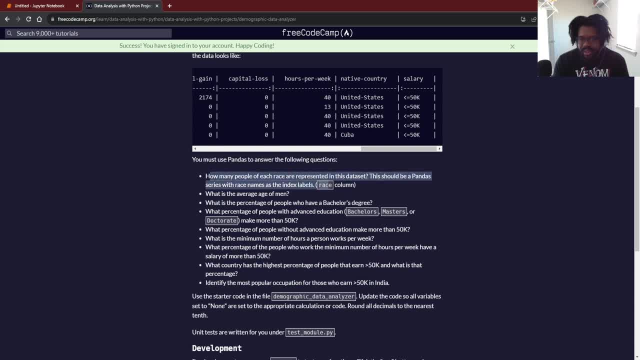 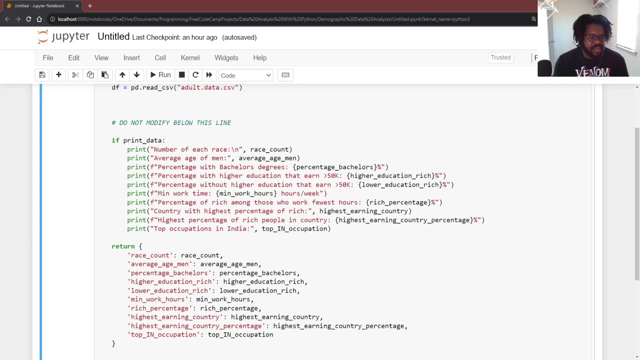 operations that we have to do for it. we're supposed to figure out how many people are represented in each race, the average amount of men, and a bunch of other stuff. so let's move over to it. i have my jupiter notebook already set up, so let me just put this to another screen so i can read the instructions, and then let's just get. 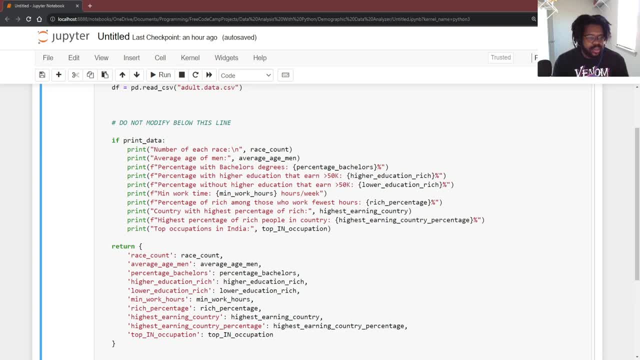 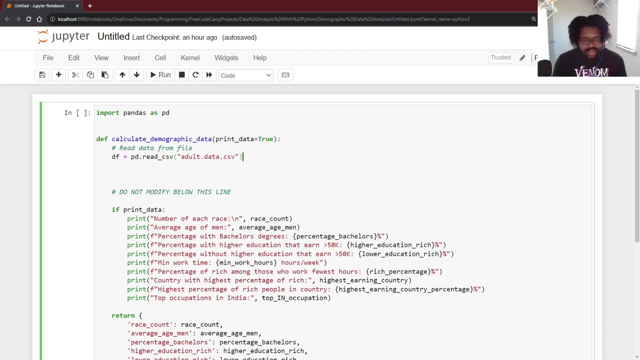 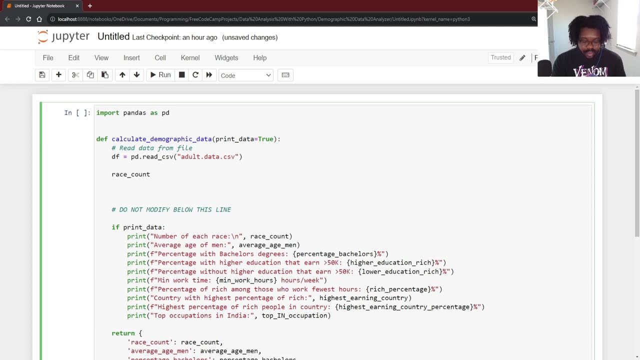 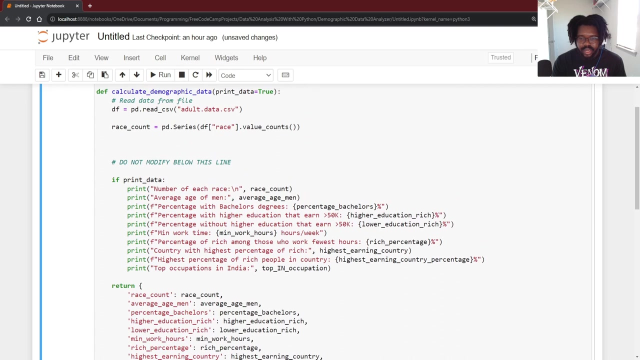 into it. so the first thing that we need to do is figure out how many people of each race are represented in the data set. so that's gonna be. race count is equal to pd, dot, pd dot, series, um, df, open bracket. race value, underscore counts and then, if we run it, we're supposed to get the races, the count of the races, the next. 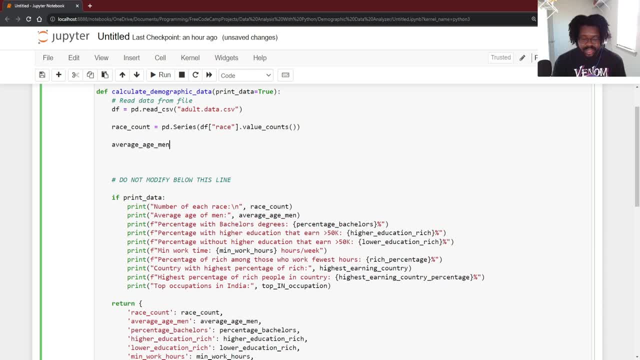 thing that we have to do is we're gonna have to figure out the average age of the men. so to do that, what we have to do is we have to first call the round because we want that we're doing the average and we want our own number or a whole number, and then we're gonna say df and then call. 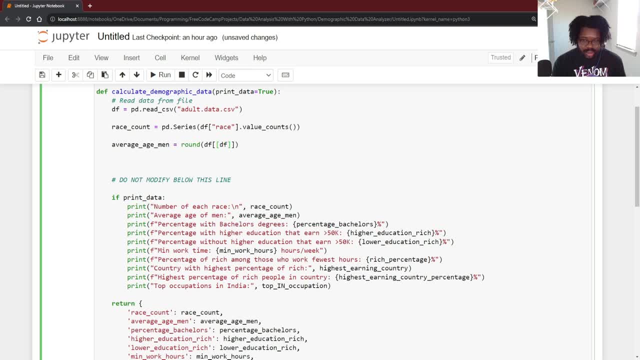 the df once more on df, df, df, boom, and then that's gonna be on sex, and then go outside of the bracket, and then for the males where the age, and then we're just gonna do a mean open that. and then comma one, because this one is for the round function, where we, um, we round it to the nearest whole number. when you done that, 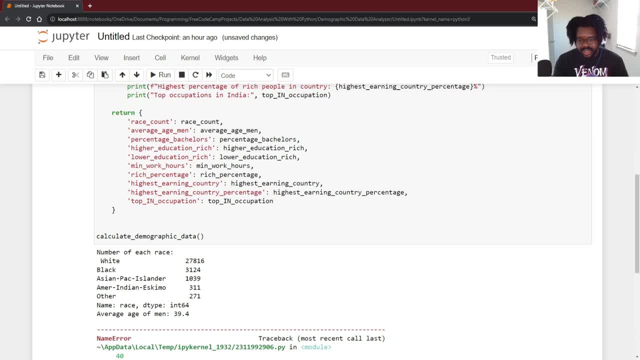 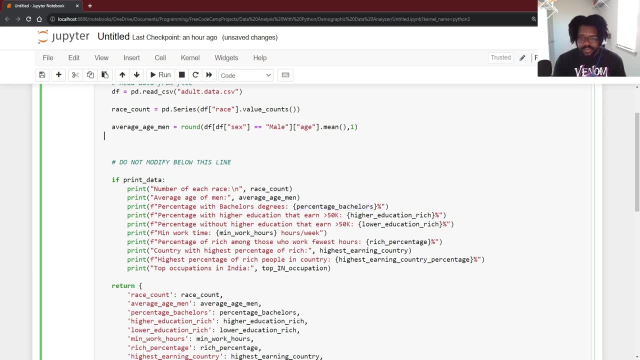 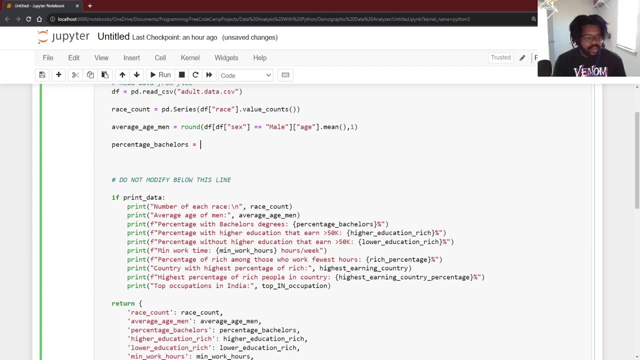 number. so if we run it, the average age of the men is 39.4. so the next, the next one we have to do is figure out the percentage of bachelors. so percentage of people with bachelors is we're doing around again and then for that we're gonna do open two brackets and then we're gonna do the 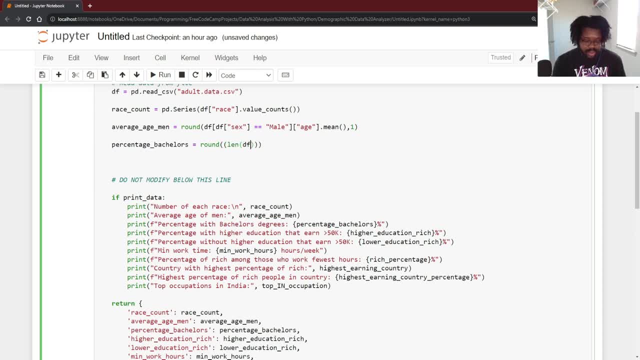 length of the data frame and then call the data frame uh, data from data education, and then equals to bachelors. and then i need to do is closed bracket it divided by the length of the data frame where df, dot, education, close the bracket twice. multiply that by 100. 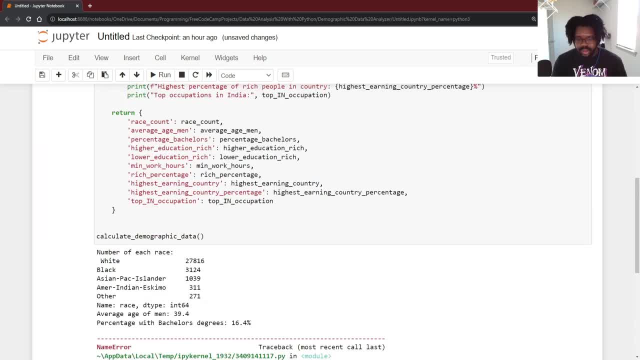 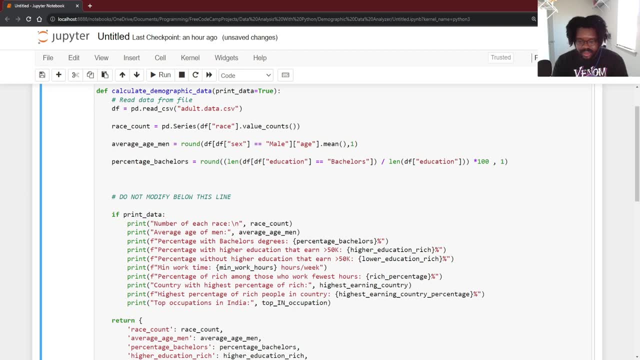 and one. so when you print it, the percentage with bachelors is equal to 16.4 percent. so the next thing that we have to do is figure out um percentage of people with um advanced degrees, so bachelor's, doctorates or masters- that make more than 50- 50k per year. so the first thing that we're 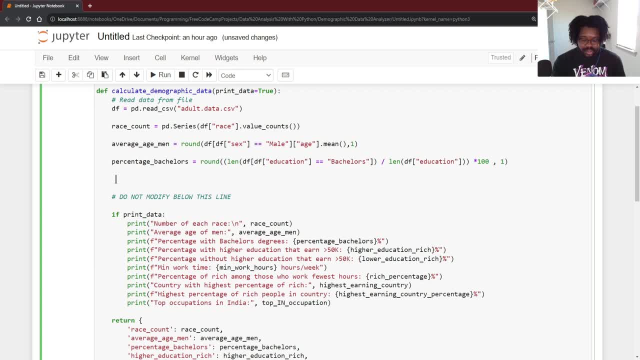 gonna do is: we're gonna just figure out, um, the number of people that have a higher education. so i underscore: education equals the length of a data frame. um, we're gonna do another and then that's gonna be df education is equal to bachelors, um. 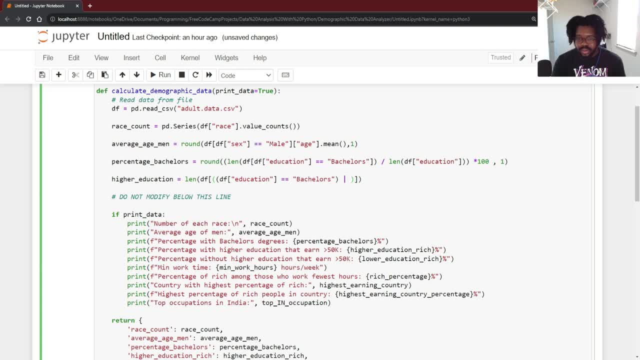 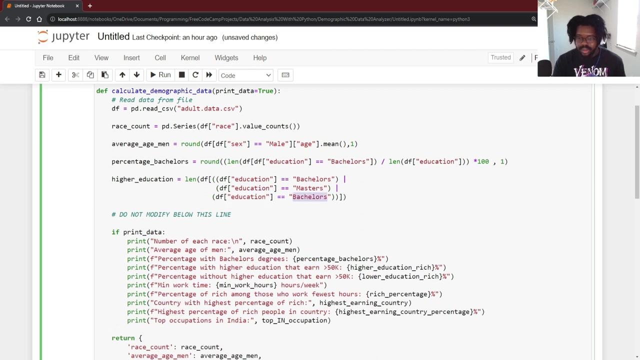 to an r, and then what we have to do is copy this after the, or paste it, change it to masters and then do another, or paste it and then paste it again, and then change that to doctor, right, and then that should complete it. so let's just make sure everything is closed appropriately. i think that's it, so let's. 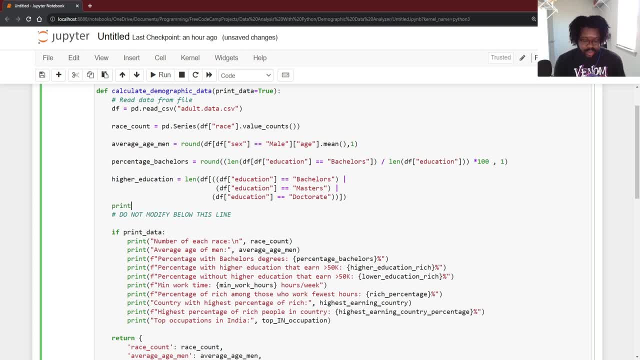 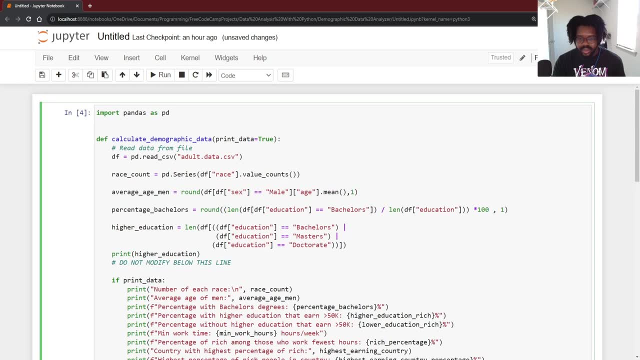 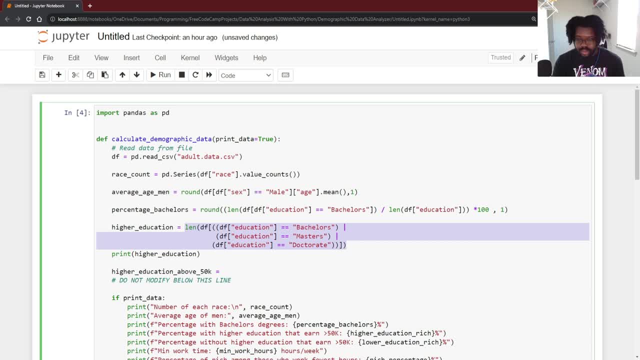 this entire thing right here, but this entire thing right here, but, but but what we're gonna do is after this, we do that and then we're gonna called and salary well, and open the bracket. df bracket salary is equal to, and then that's going to be greater than 50k and that should complete it. 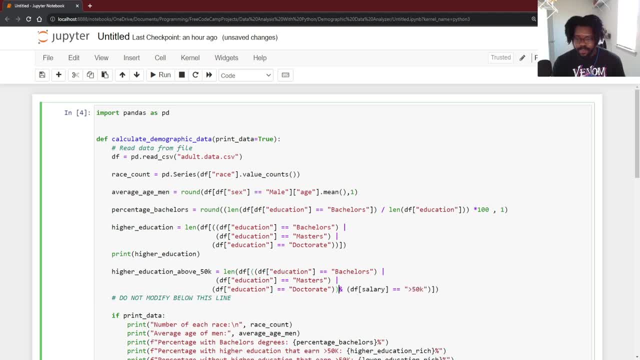 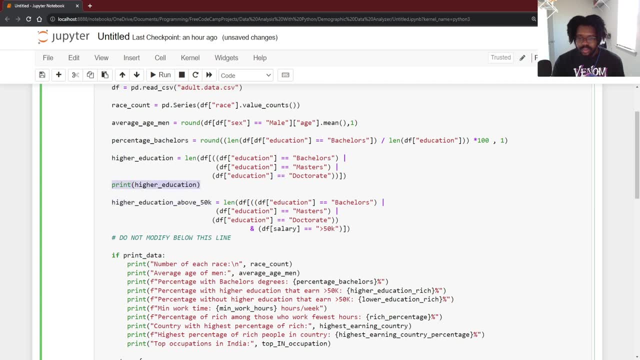 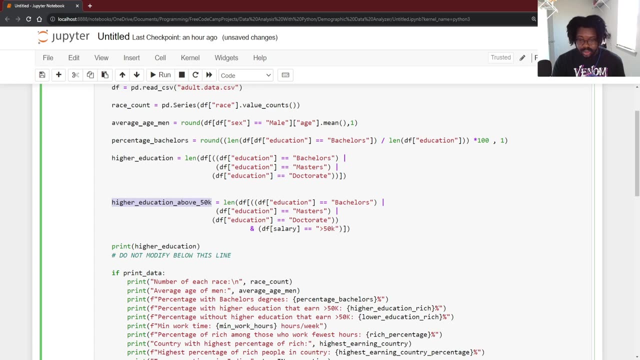 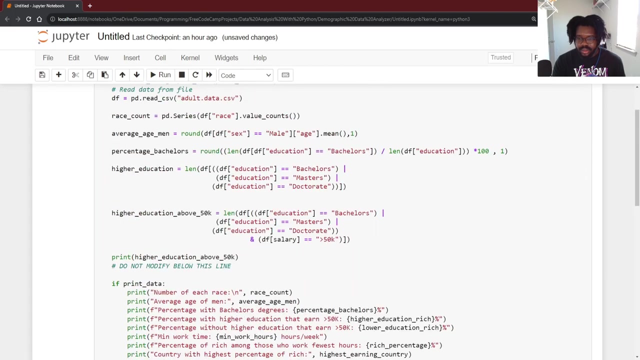 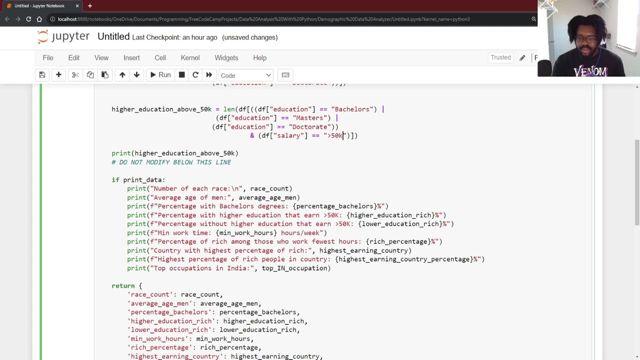 i guess, and then let's just do a print on that as well, just to make sure it seems right okay, and salary is not okay, so that's because, and then we're getting zero, so that's an issue, and that's because it probably exists as a capital. 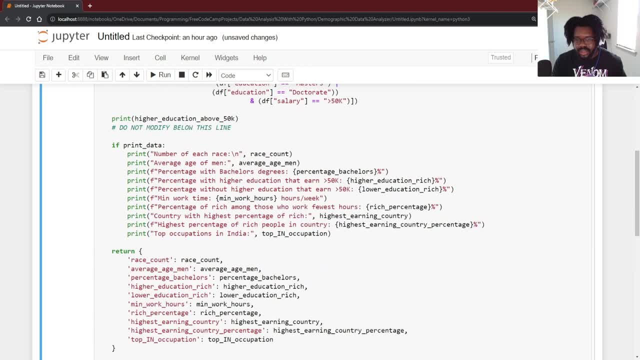 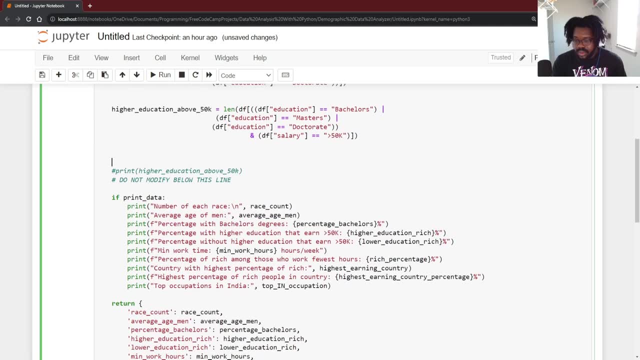 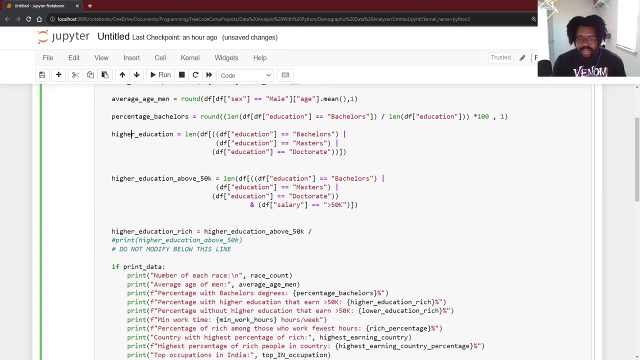 k, so let's run it. we have 3486, so we can just comment out the print right here and then i'll all we have to do is just do the percentage, which would be- uh- i believe it's this- divided by this, and then multiply that by 100. so what i'd have to do is copy um, close that into. 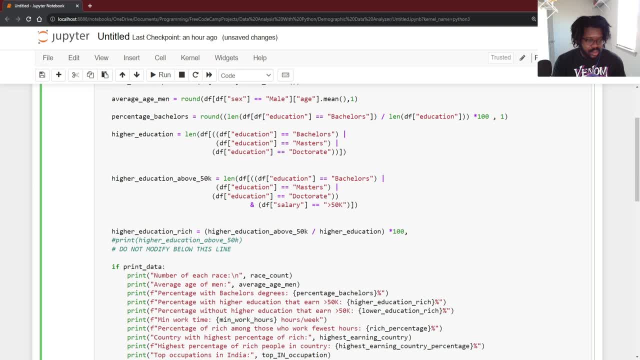 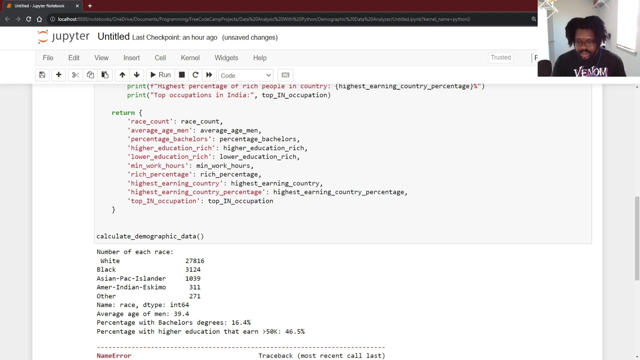 a bracket, but we want uh round to the nearest whole number. so that's one. so that's probably close that again and then that would be round, i believe. uh, it would be over here and if i print it it's 46.5. so the next, the next. 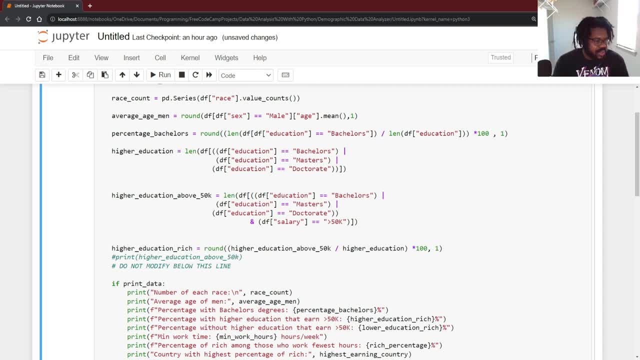 instruction is: what's the percentage of people without advanced education that make more than um 50k? so still greater than 50k, but they don't have advanced education. so let's do just copy that. so it's essentially the same thing. so i do that. 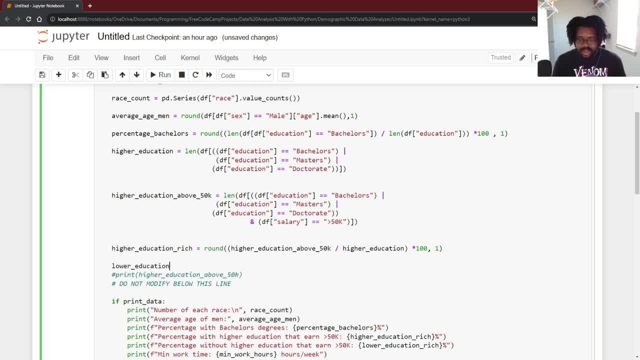 i'd name it lower, i'd name it lower education, and then that's this, and then i'll just copy this again: and instead of equal, we have not equal, and not equal, not equal, and then, and then i guess i could change these to: and, but would i need to? i'm not sure, because if it's that, 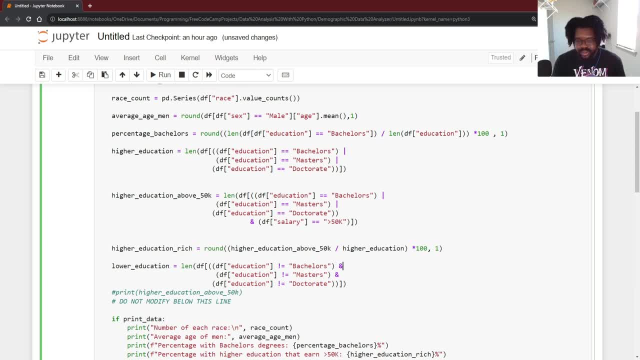 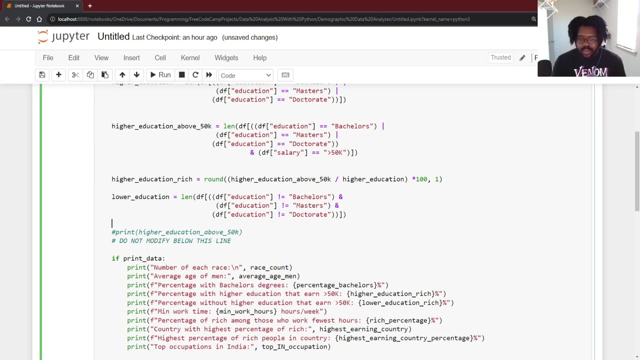 or that, or the length of that, or the length of. okay, let's just do. and so wouldn't this be the same thing? oh no, because it would probably have all of them. okay, okay, all right, cool, cool. so, with that being said, that should cover it, but let's just do a print on it nonetheless. 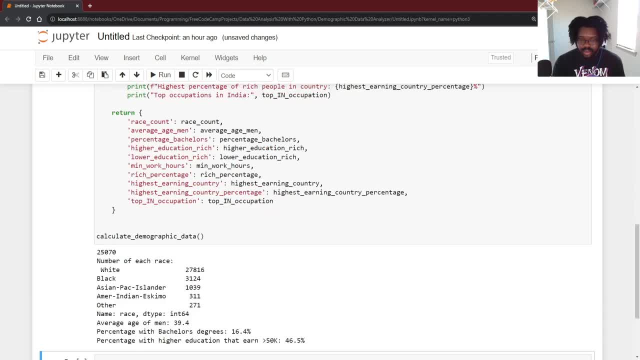 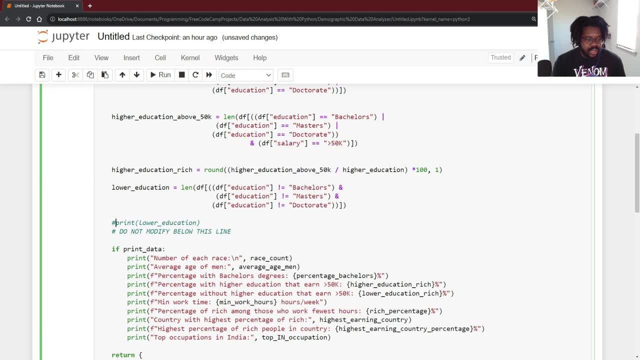 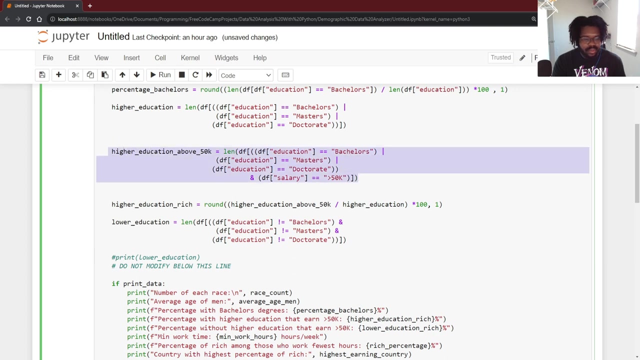 let's see if we got a value 25 070. so we do have a value, but they need to make and we need a percentage of without advanced degree that made more than 50. so it's the same as this. so all i'd have to do is just copy this. 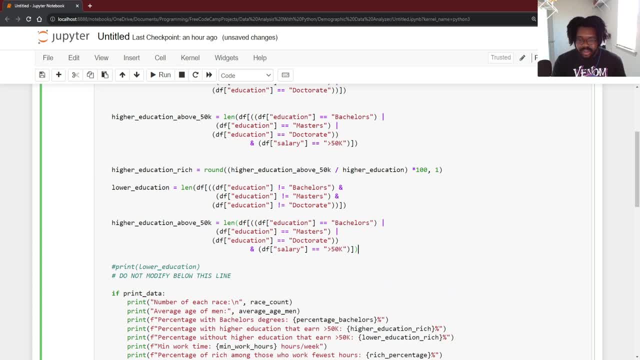 paste that there. lower edge. no, that's the wrong one. um, let's do lower education, and then not equal to, not equal to, not equal to, equal to, and then i guess these would be ants also, and then, if i run a print on this, we have a value of 4355. 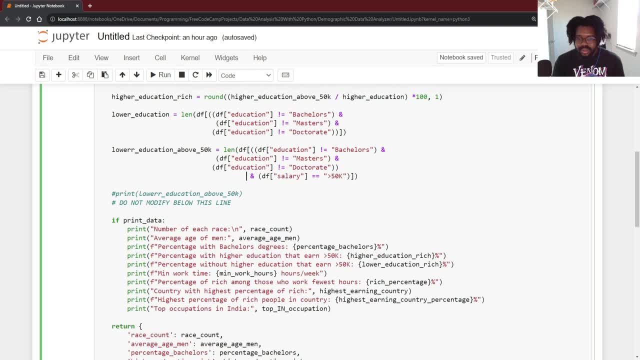 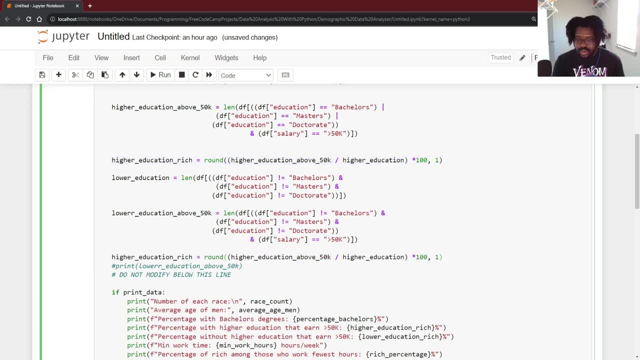 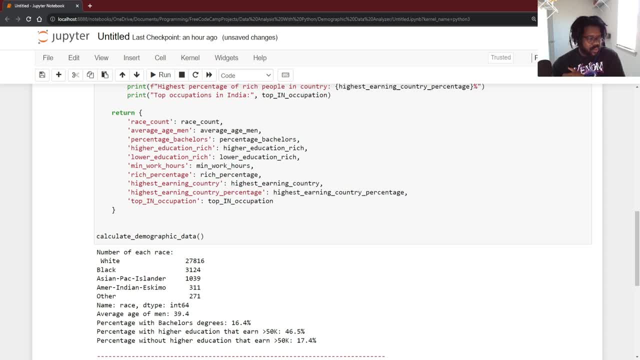 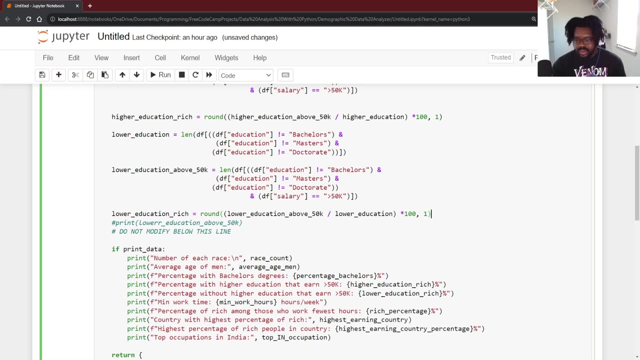 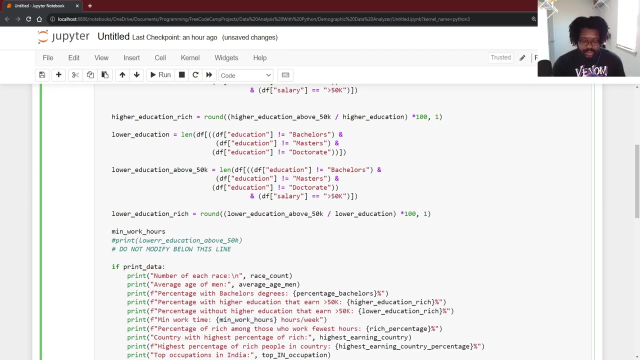 four percent. so the next question that we have to do is: what's the percentage of beef? so what is the minimum number of hours a person works per week? so to calculate that, one minimum hours per week would be equal to DF open bracket, and then that'll be hours per week, and all you have to do is just call the min. 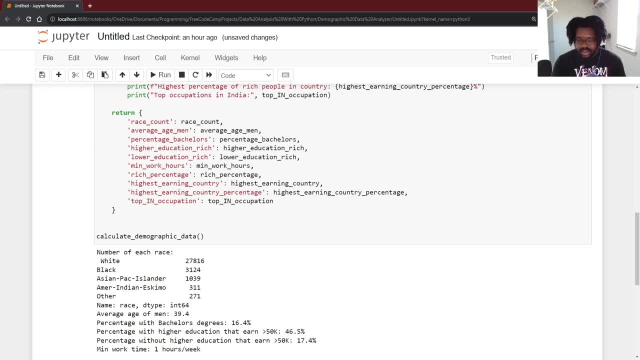 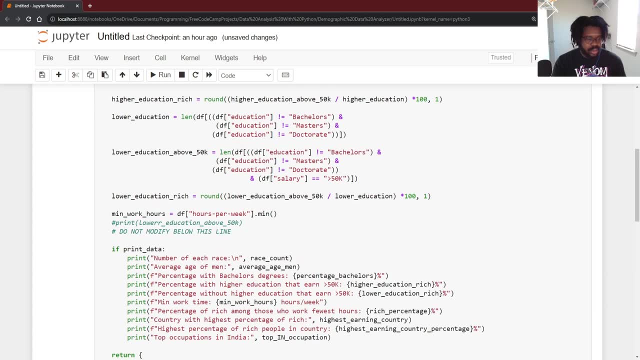 on it and then that should suffice. so minimum number of weeks is one hour per week. yeah, and then the next question is: what is the percentage of people who work the minimum number of hours per week, have the salary of above 50k, so the minimum hours per week and they have a salary above 50k? 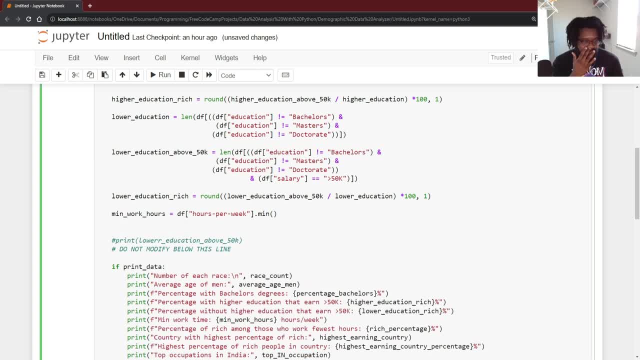 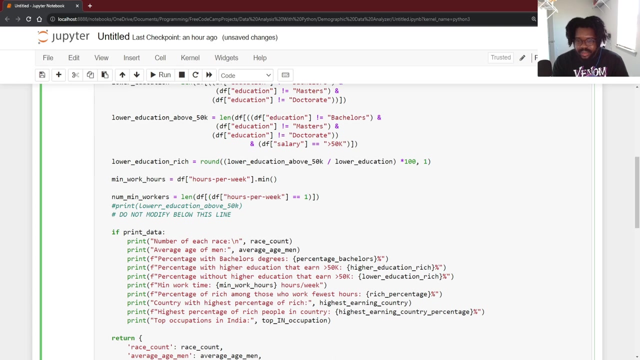 so let's first let's do number of minimum hours per week. so let's do number of minimum, and that's gonna be lent bracket, then that's gonna be equal to 1, so that's the length of everybody that works the minimum hours per week, which is 1. 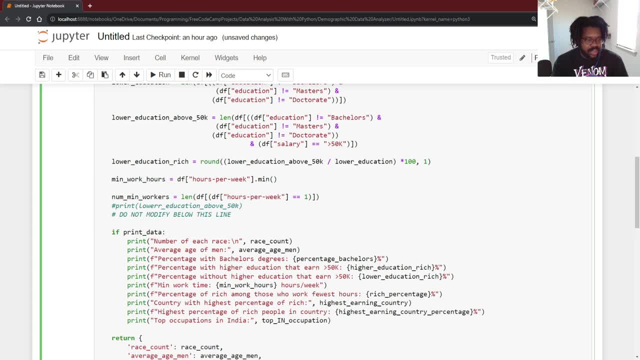 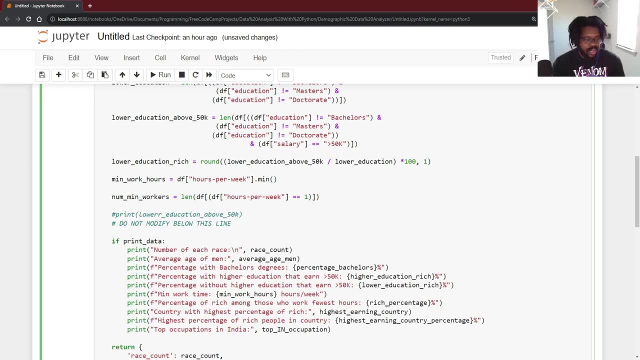 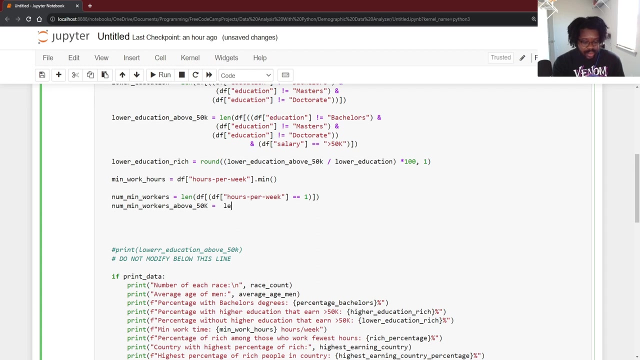 right, and then now what I have to do is get those that work it and make more than 50k, so let's call this one num minimum workers above 50k equal, and then be length time- well, not times, but length of the data frame, of the 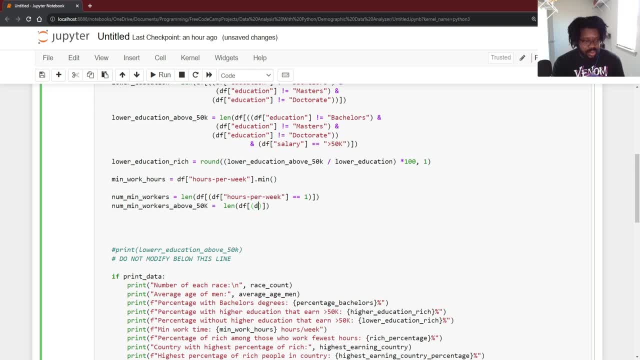 data frame, df, and that'll be this piece of thing right here. copy that equals minimum with ours, and df salary is equal to 50 k. 50k and then has to be greater. so the length of the data, the length of the data frame of those that work. 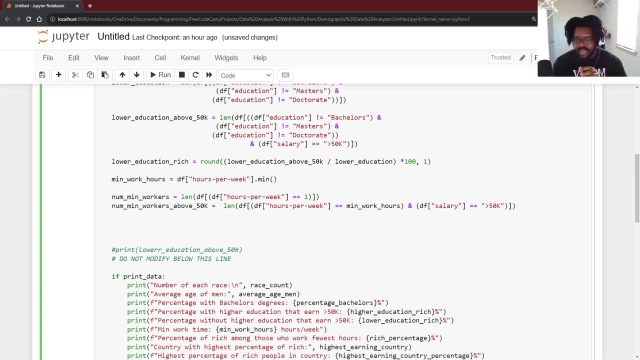 the minimum hours per week and their salary is greater than 50.. and then I guess we just divide them both, so let's just call it the rich percentage. so the percentage of rich among those who work few hours. yeah, so that's gonna be equal to: I believe it's. 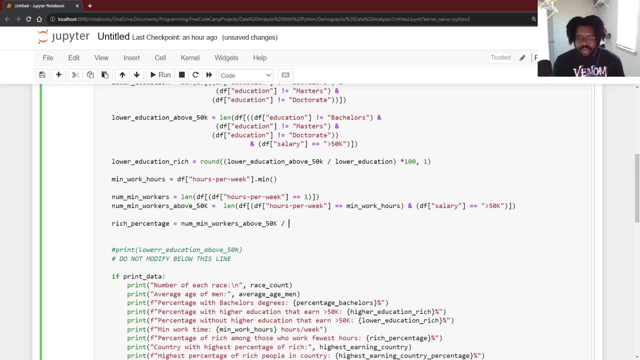 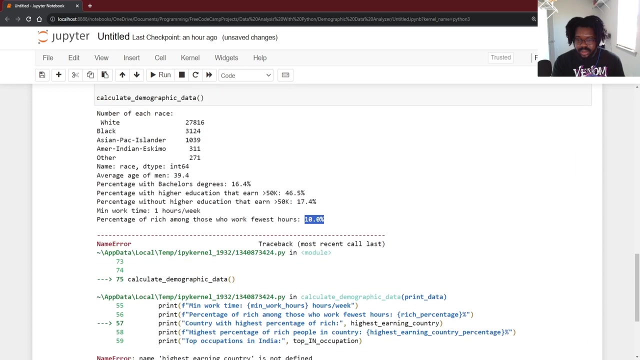 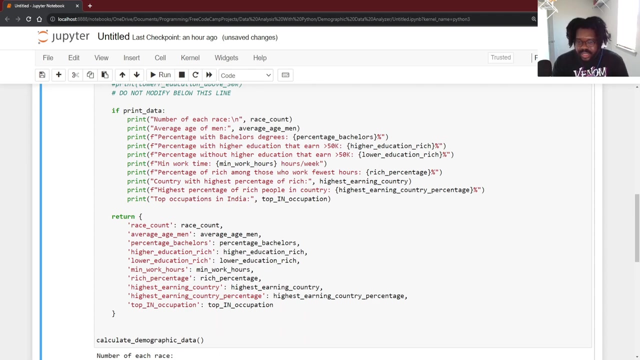 this divided by this, then wrap it into a bracket, multiplied by 100, comma by one, close the bracket and then browned, and that should give us our total, which is 10 percent. so the next one is the country with the highest percentage of rich, the country the highest percentage. 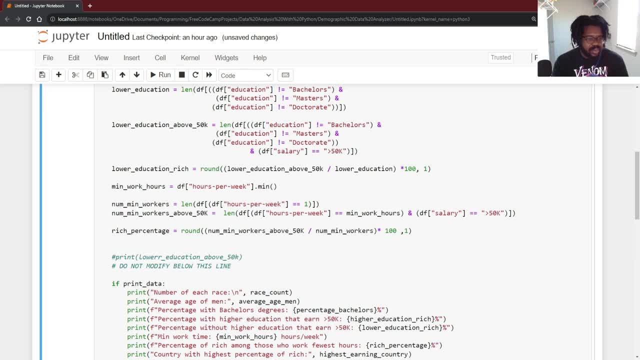 of rich. what is the percentage of people? what? what countries has the highest percentage of people that earn greater than 50 and what is the percentage? so that's a two-part question. so first I have to figure out which country has the highest percentage of people that work more than 50.. so 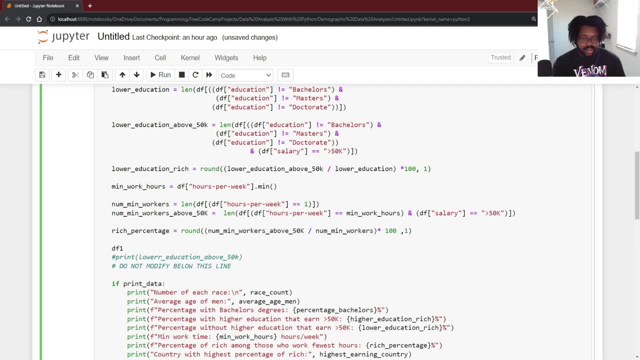 that would be. let's just say df1, df1, and then let's just go around and then again: df- open bracket, open parentheses. df- dot salary is equal to greater than 50k, then close the bracket and then close the. we'll close the percent parentheses, close the bracket and then get the native country. 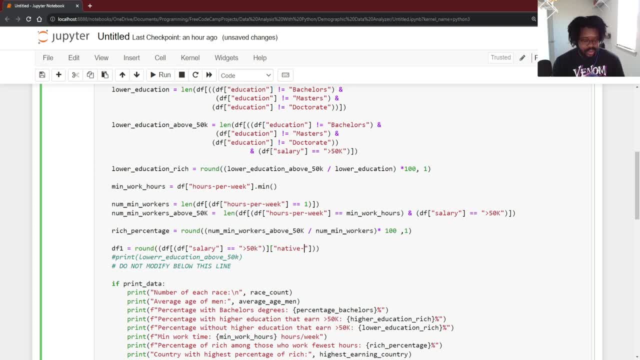 value counts. well, not native, but country value counts, underscore counts, open the bracket and then we divide that value count by the df. are the entirety of the um, native country, native country, rather, native country, dot value, underscore counts, and then that's close, close, close and no. close that, and then let's do. 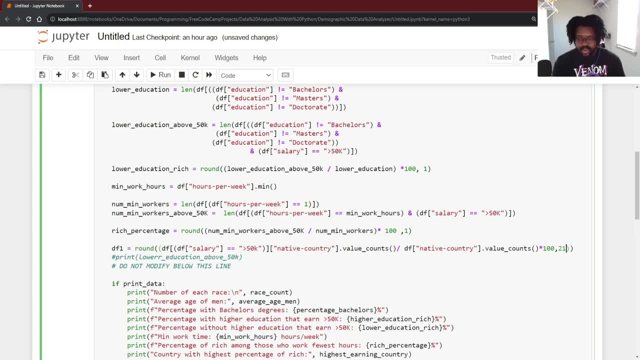 times 100 and that'll give us one. so what this is, what this is doing, is so we get the salary of those with the highest um, with above 50, and then filter by the native country or a group by the native country, and then we get the value counts and then we divide it by 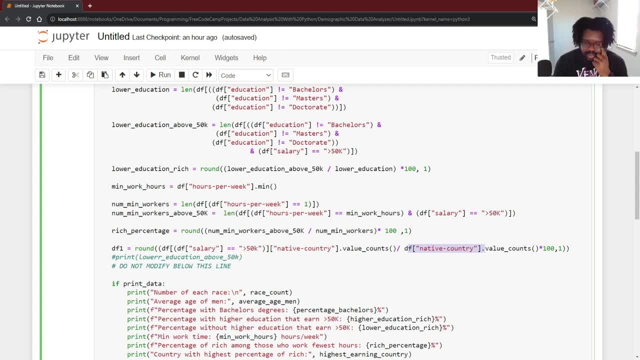 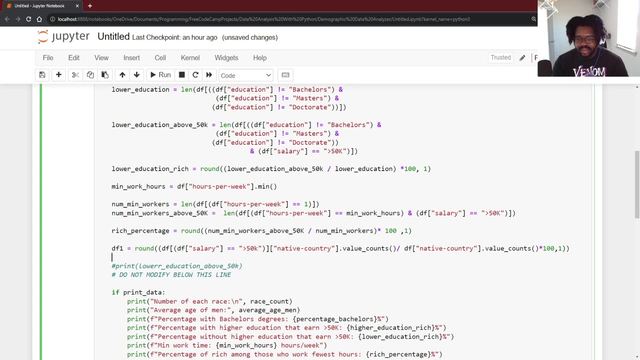 the native country. so that would give us the percentage, and then what we have to do is: so that's for the entire data frame, so we get the salary of everybody that's above 50- 50k. then we group by native country, where we have the value counts. 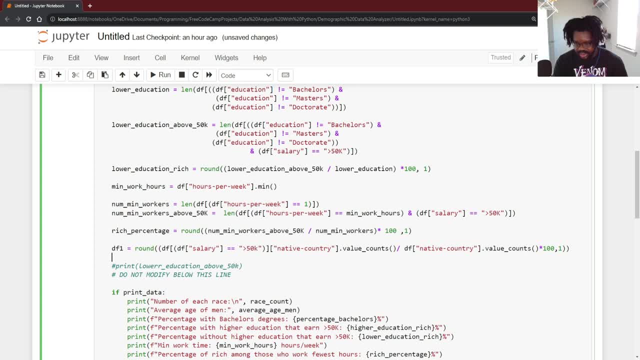 so we group the value we get the value counts on group by the native country and then we divide by. we divide by the native country, value counts. so that's going to give us percentage and what we have to do is just sort it by one. well, not sorted by one, sort it by ascending. so it's tf1 dot sort. 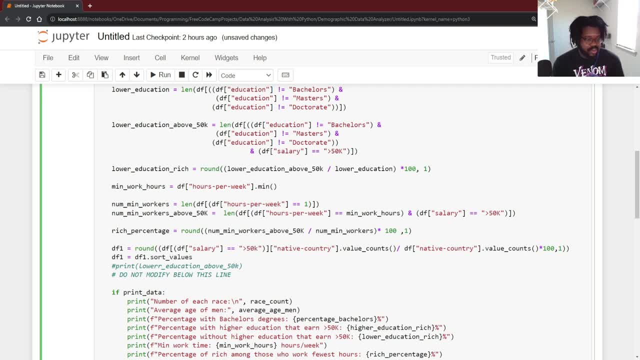 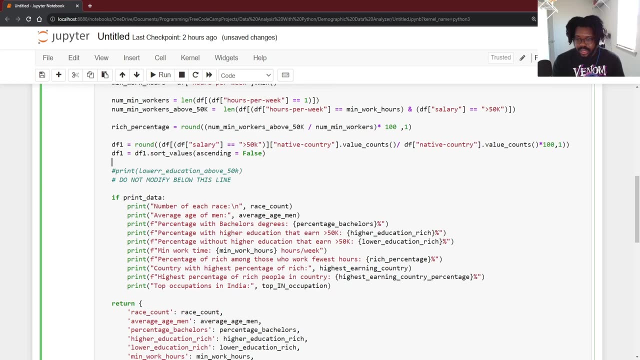 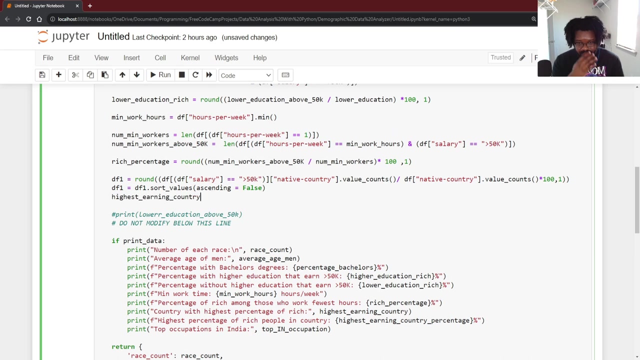 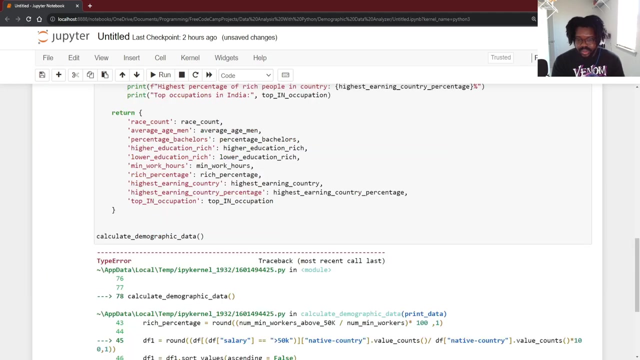 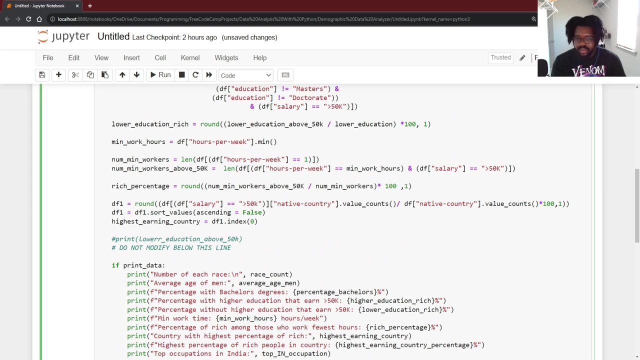 underscore values. ascending is equal to false, and then the highest condition would be obviously, well, starts from descending. so largest to smallest, so the highest country would be at the very first index. so that's tf1, dot index zero, and then that should give us our country. but something was wrong. top of the find round method: round method. 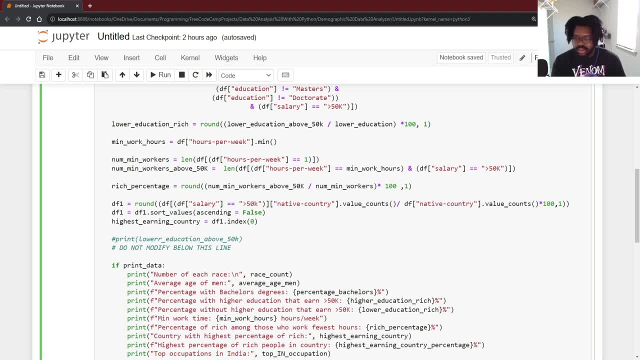 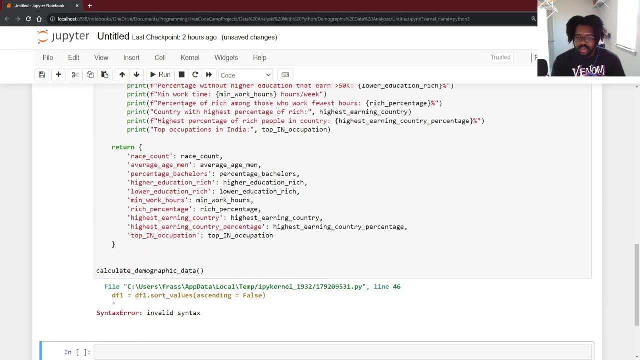 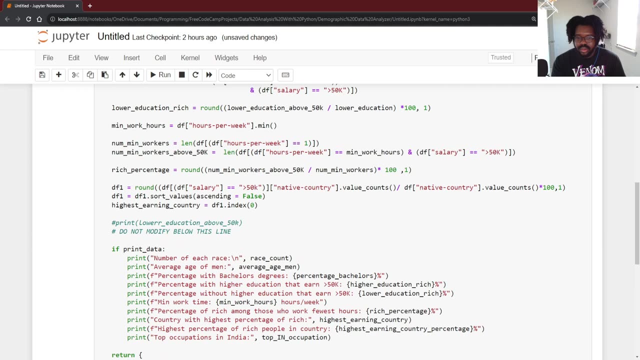 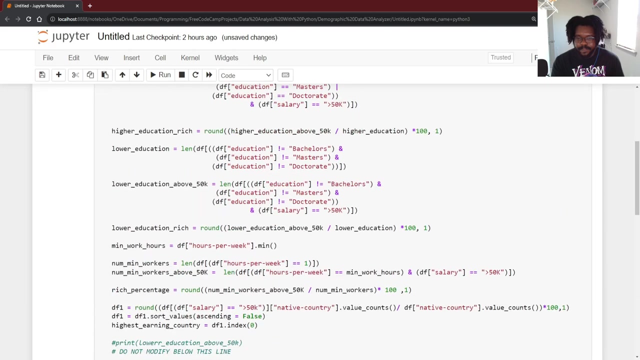 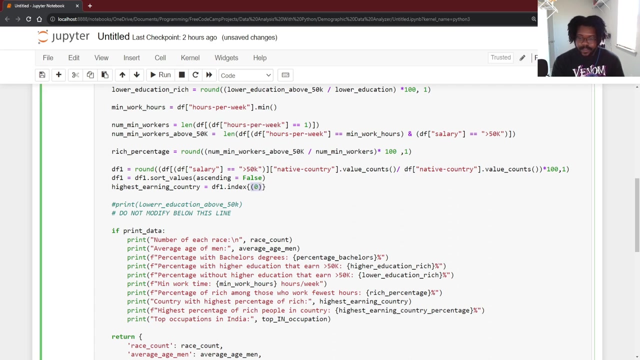 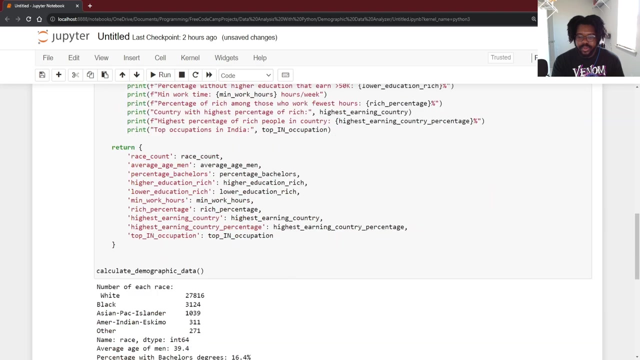 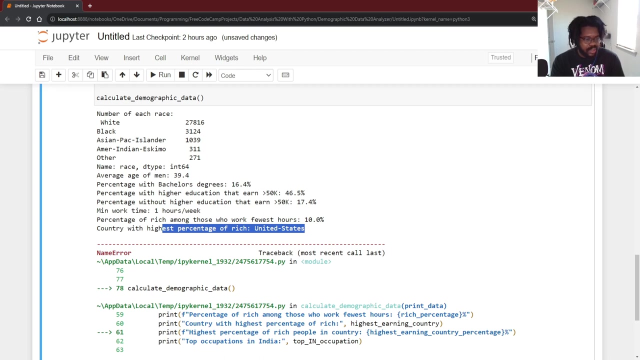 so something is: let's see, nope, invalid syntax, df1, so i guess i didn't close it. yep and close it. well, actually it doesn't close there, it closed here here, and then index is not callable. sorry, there we go. so the country with the highest percentage is the united states. 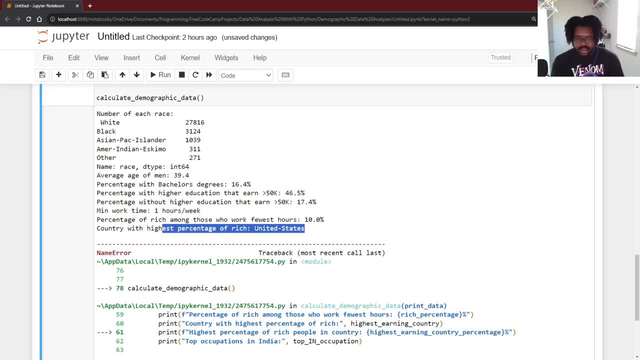 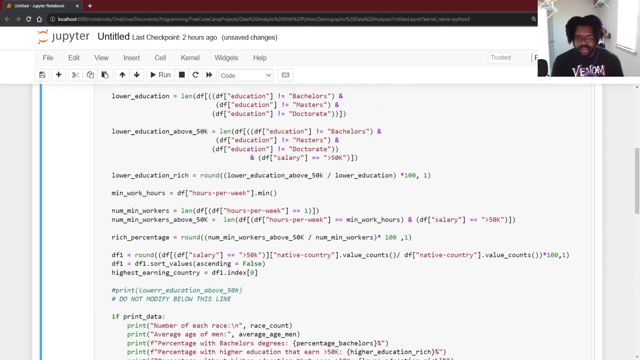 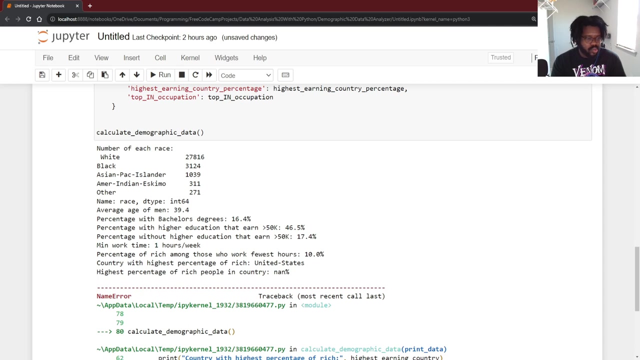 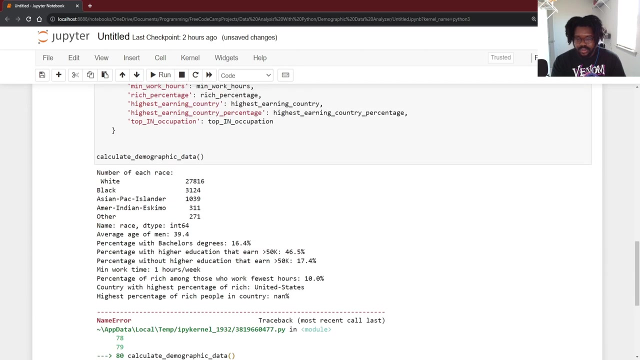 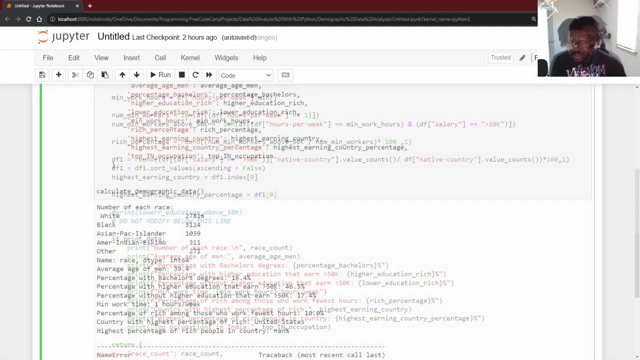 the highest earning country. okay so, and then we need the percentage. so then all that would be is equals one and let's just call the value. that's not index zero and that's inaccurate to say the least. all right, so we figured out the reason why this is: give us not giving us not a. 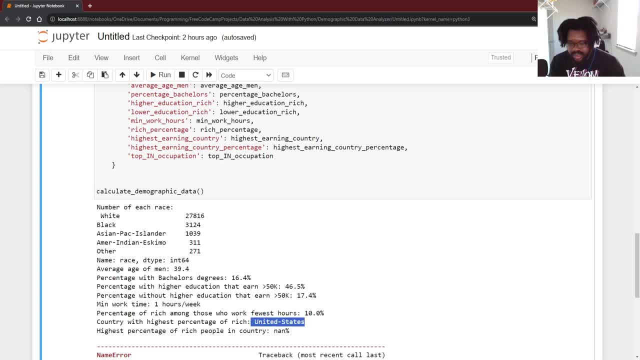 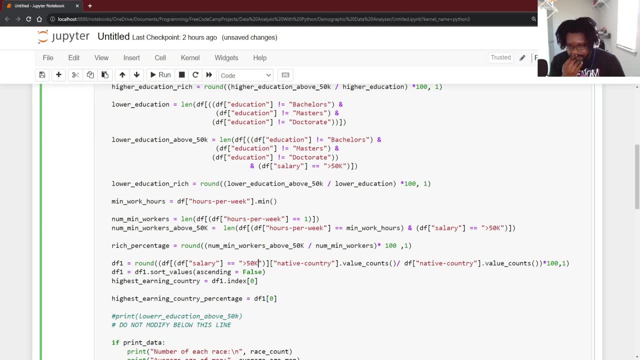 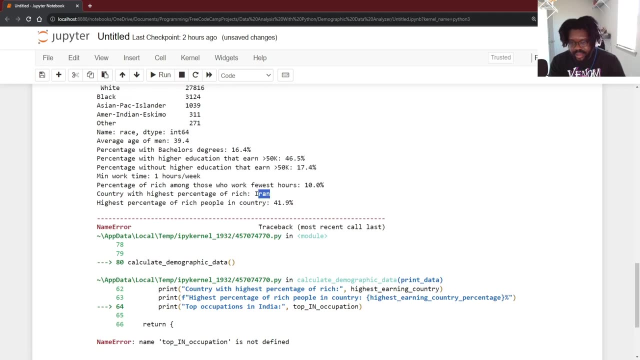 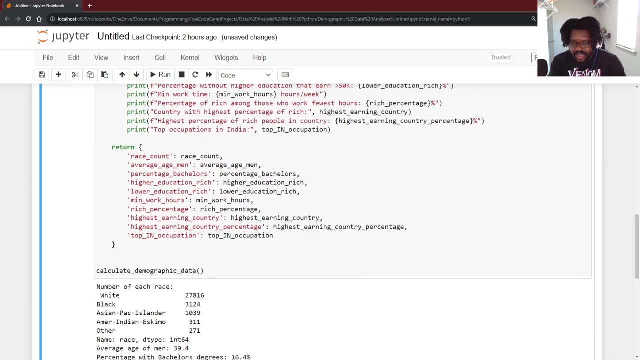 number and, as a result, because that this is also incorrect and that goes back to this right here, it's not 50k lowercase, it's 50k uppercase. so if we do it again, you, we should get Iran, with the highest percentage being 41.9 percent. so then, 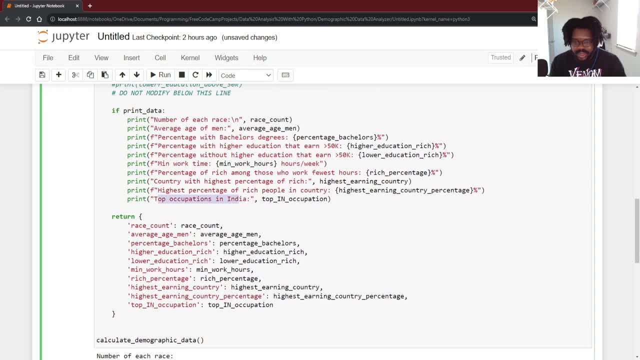 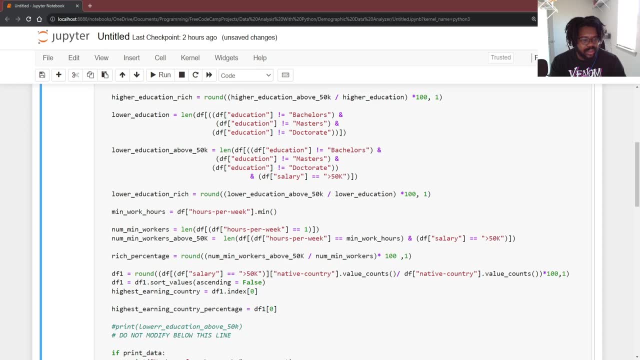 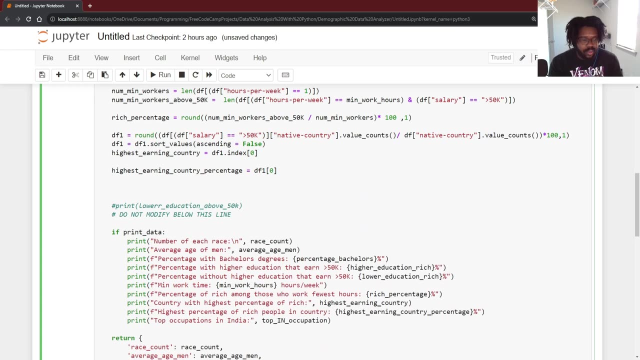 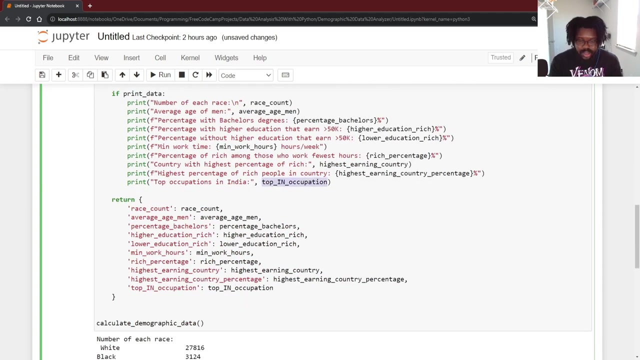 after that, the last one that we have to do is the top occupations in India. so, top occupations in India, that's gonna be. let's just say that we should get Iran, with the highest percentage being 41.9. let's do, yeah, let's just copy this, paste that. 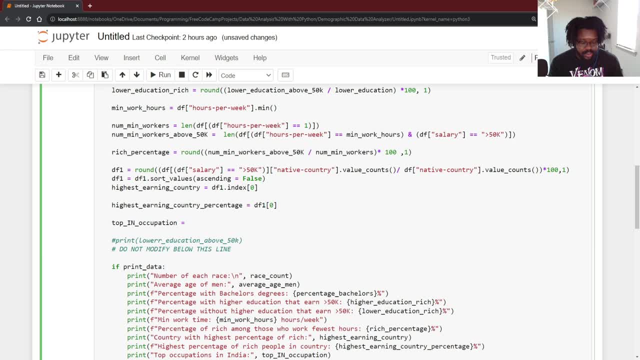 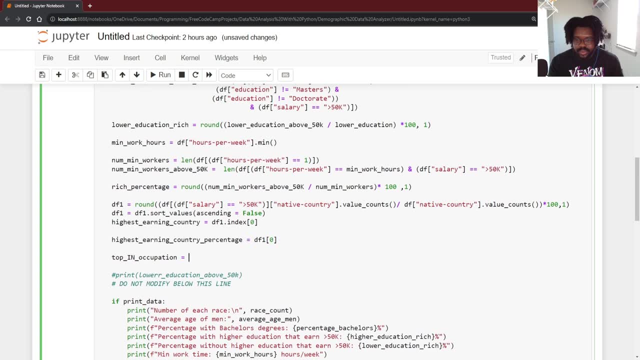 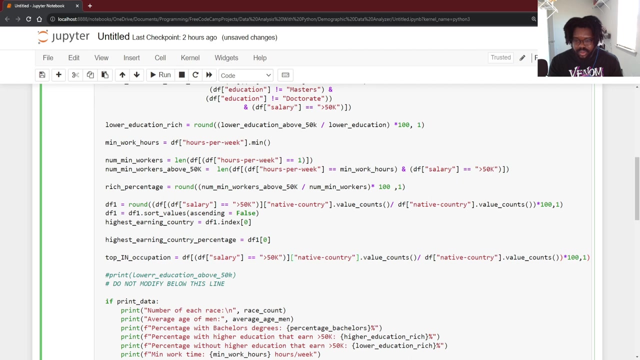 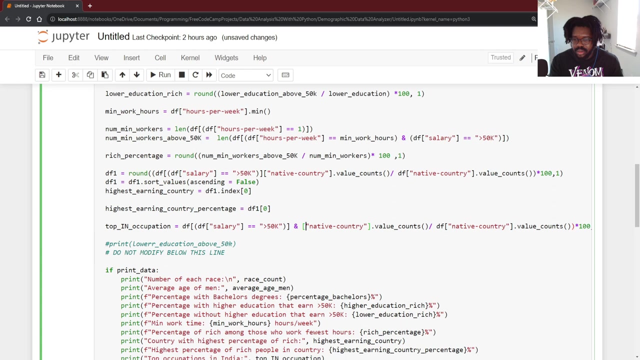 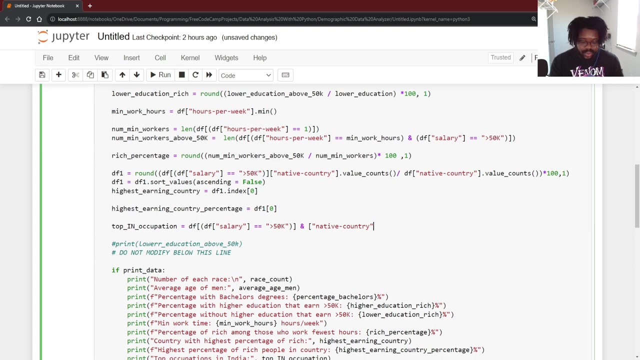 and then is equal to: let's go. actually, all I have to do is kind of copy this a little bit. then: 50k Grams, Okay so 50k Grams, 50k, native country, 50k and the native country, so data brief with the salary. 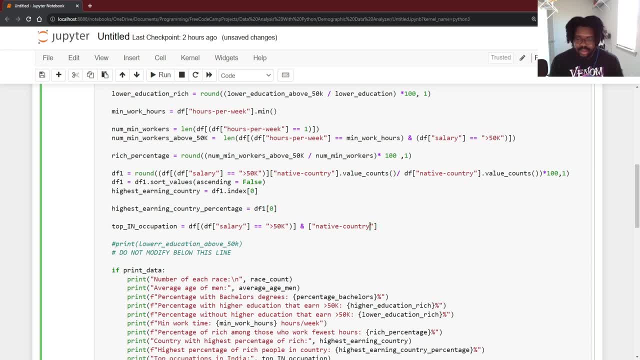 about 50 key and the native country. put that into parentheses. native country is equal to India. yeah, native countries equal to India. closed that. let's see if it needed to be closed. that cost us. never needed that one, so we're getting where the salary is greater. 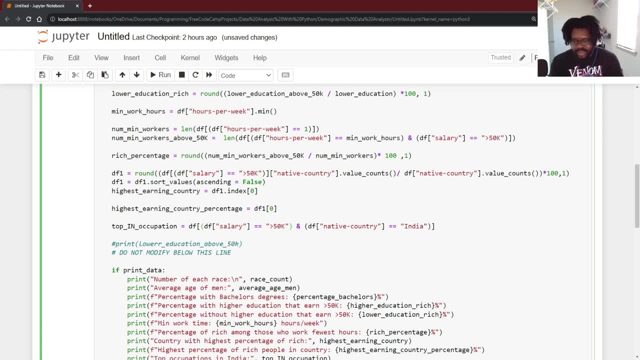 than 50 and the native country is in India, because what we have to do is get the top occupations in India right, So the occupations that pay more, um, and then we need to do is open another bracket and then occupation. uh, value counts, goes bracket dot index. 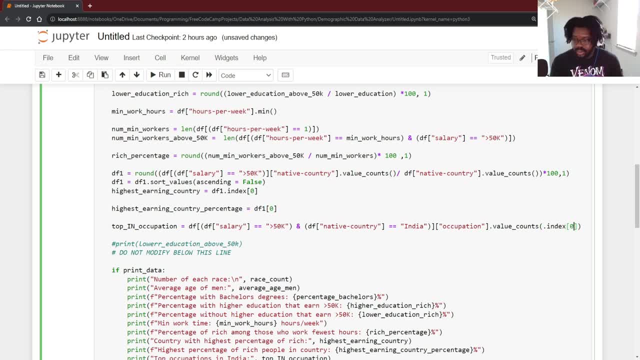 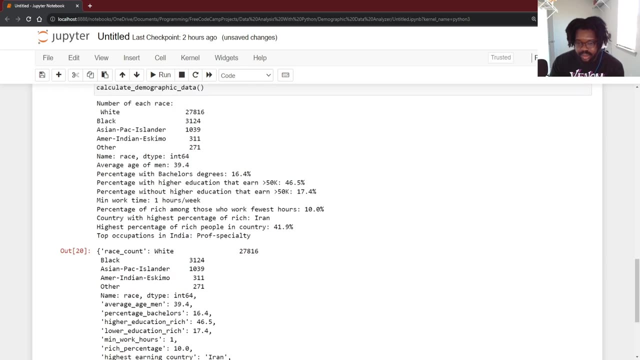 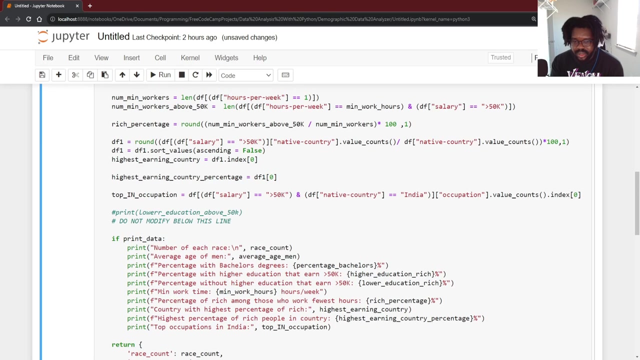 And then there we go along, sorry, getting the one that's at the highest index and that's gonna give us prof speciality or specialty, whatever that is. So let's go over it. It's the top occupation in India, where so we have to get. 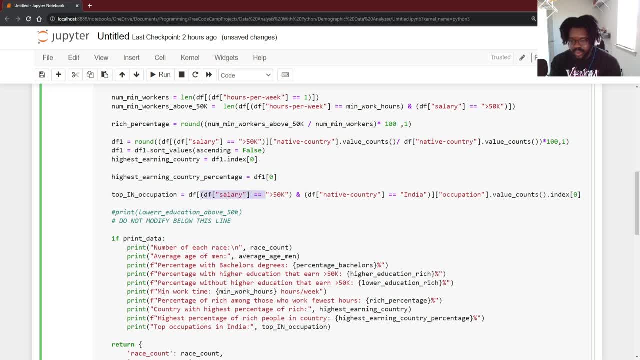 We have to get the salary above 50 K and native countries equal to India, And we grew wide occupations and then we just get the value counts and then, whatever it is, that's at the first index, That's the highest one, I believe. 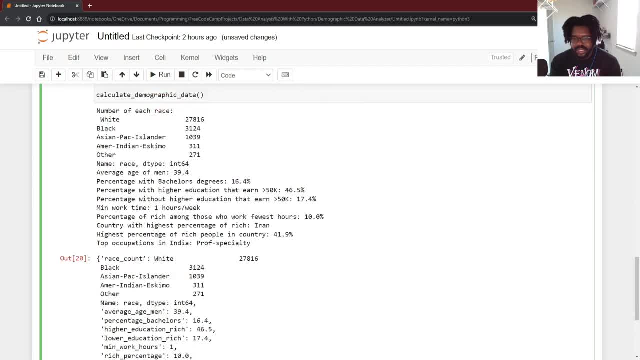 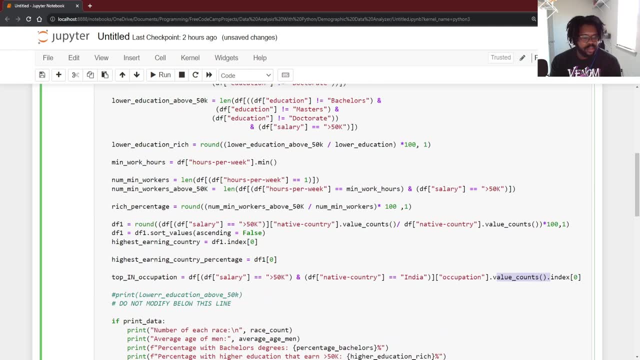 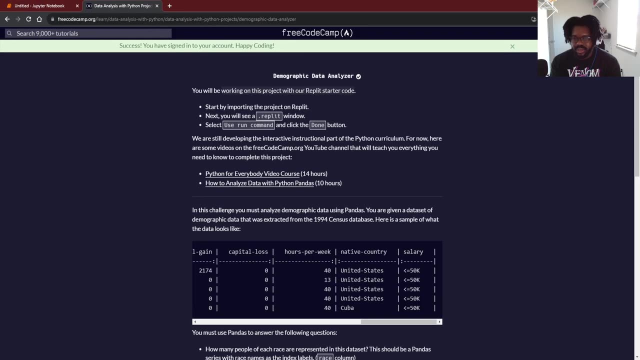 Yep, And then that's it for the entirety of Okay The project. So what we do is we just click on the replica code and then we just copy everything over and paste it in, but I'm not going to do that. So that's how we do the demographic data analyzer.